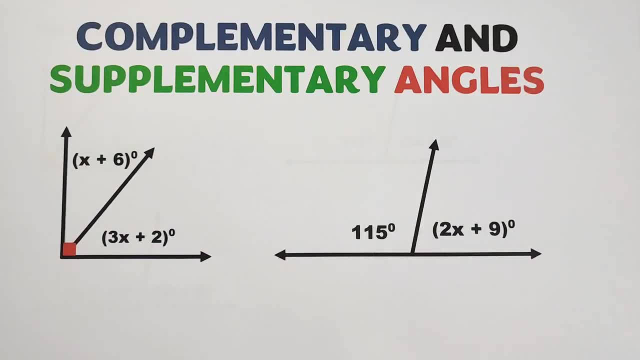 Hi guys, it's me, Teacher Goen. In today's video we will talk about the part 2 of our topic, Complementary and Supplementary Angles. This time we will incorporate algebra in solving problems regarding to geometry. So, without further ado, let's do this topic. So here are the. 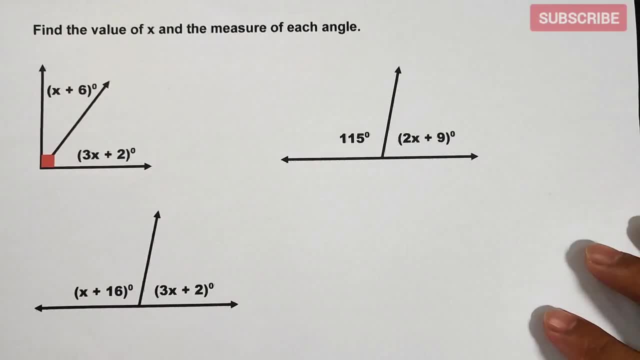 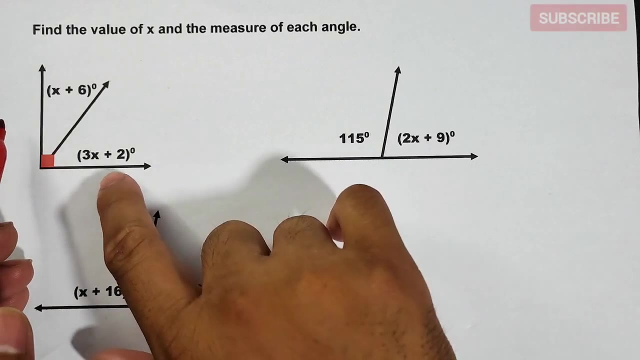 questions or the problems for this video. We are asked to find x and the measure of each angle. So, as you can see, I have here three different figures wherein some of the angles here are represented by algebra expressions. Let us try to solve this one. As you can see, 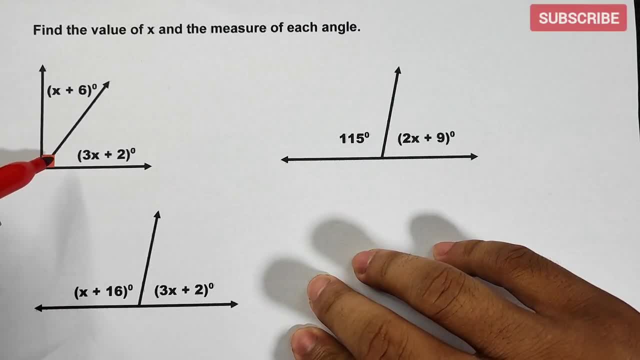 the whole angle or the bigger angle here is a 90 degree angle, meaning we can use the concept of complementary angles, because this angle- angle 1 and angle 2, are parallel, forming complementary angles. So how are we going to solve this kind of problem? 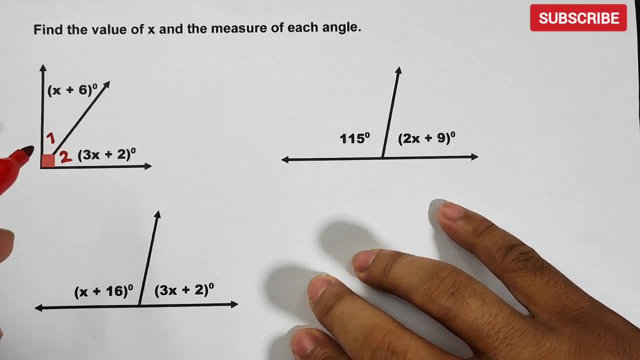 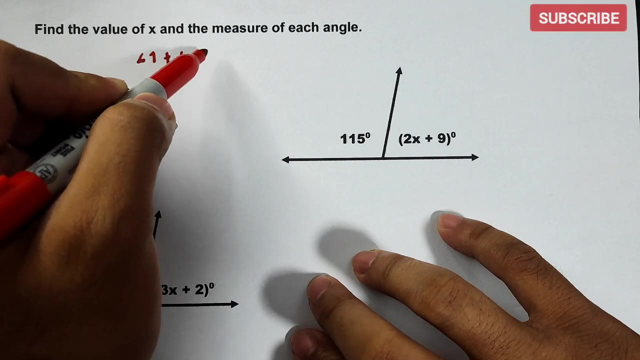 Since they are complementary. the concept is that if the two angles are complementary, meaning the sum of the two angles is equal to 90 degrees. So to solve this, let's create first an equation. We have: angle 1 plus angle 2 is 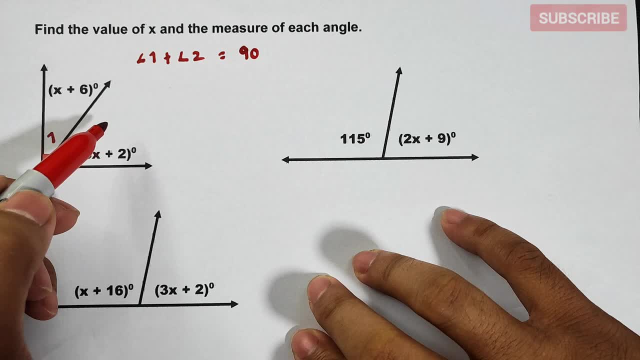 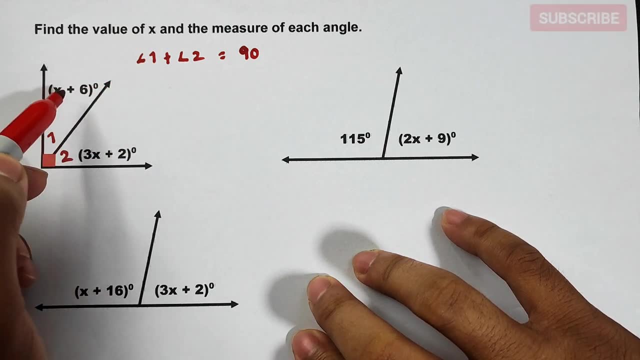 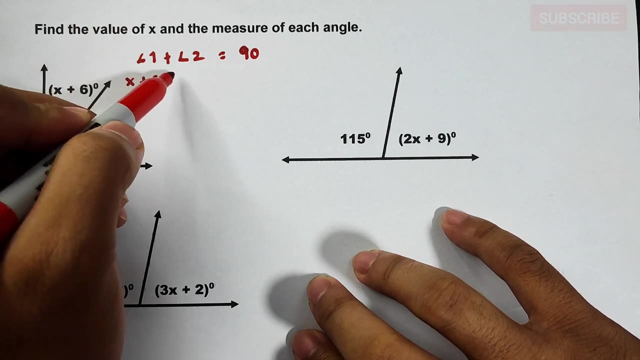 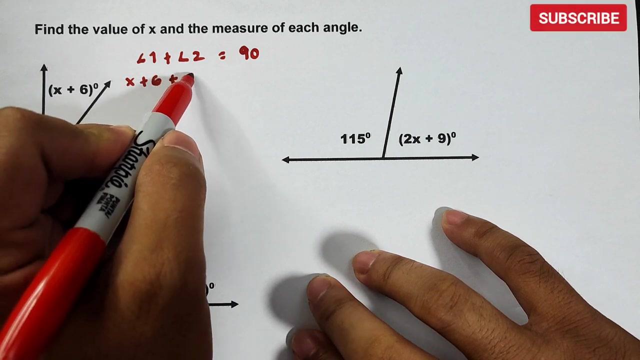 equal to 90 or 90 degrees, Then let's use the expression here represented by this one. Your angle 1 is represented by x plus 1 degree, x plus 6 degrees rather. So let's have x plus 6 plus your angle 2 is represented by 3x plus 2.. We have 3x plus. 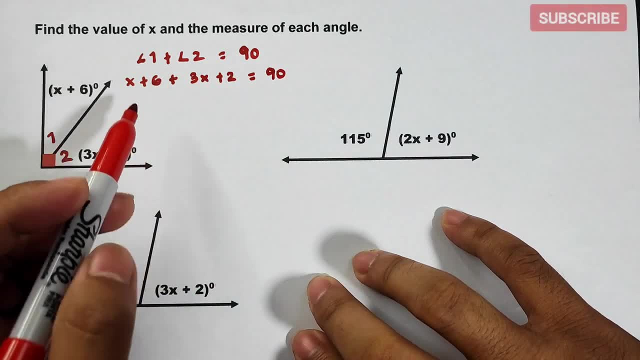 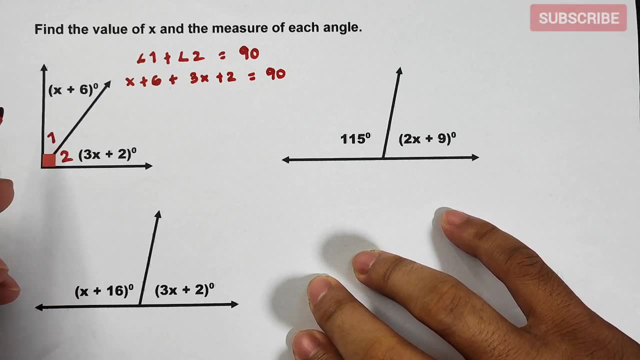 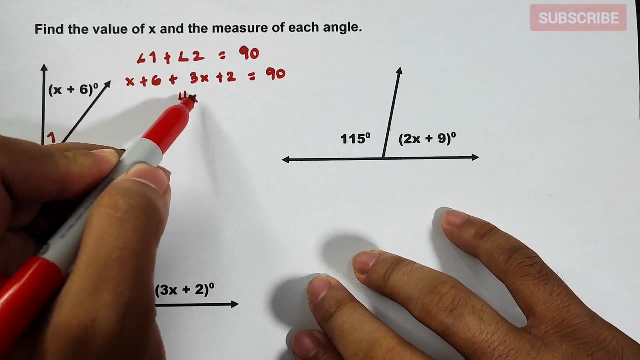 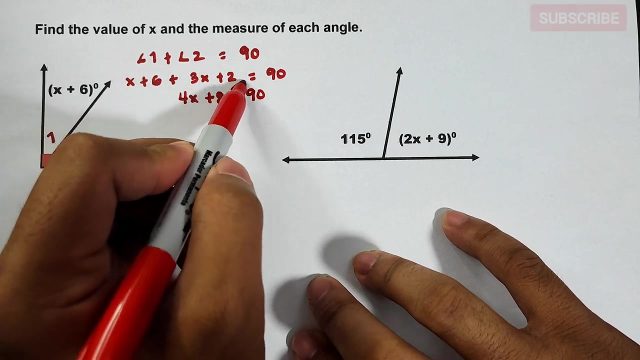 2 is equal to 90.. Our first thing, the first thing we need to do here, guys, is to solve for first for the value of x, for us to find the measurement of these two angles: x plus 3x is 4x, 6 plus 2 is 8 is equal to 90.. Transpose 8 to the other side, it will. 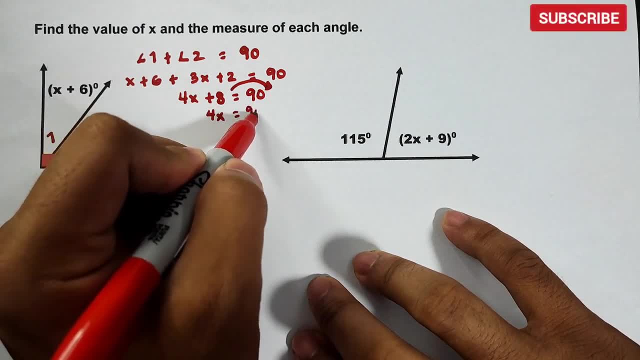 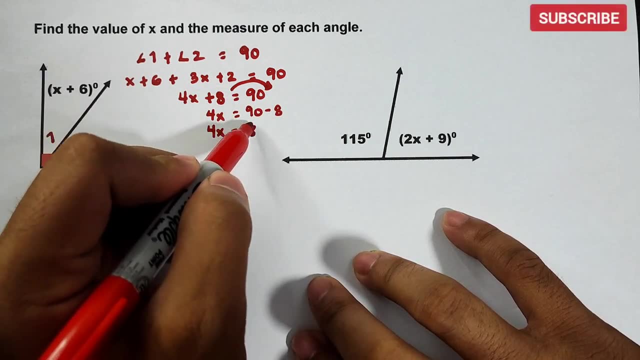 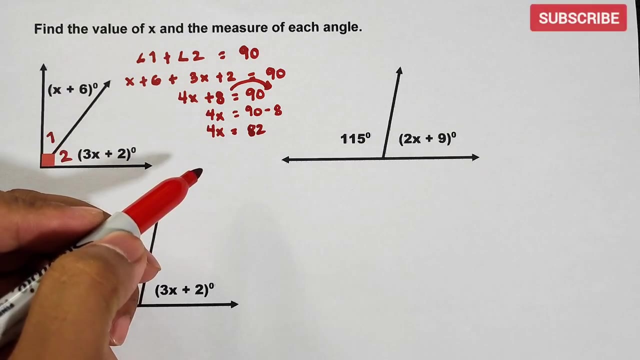 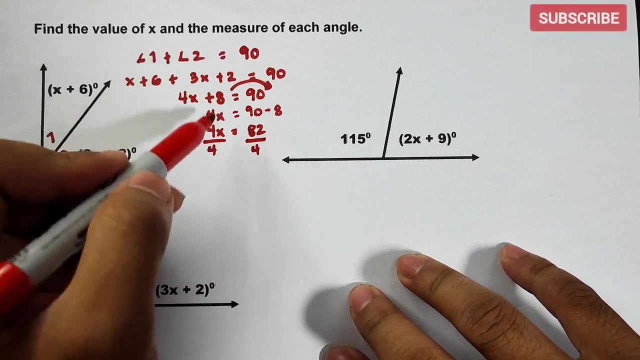 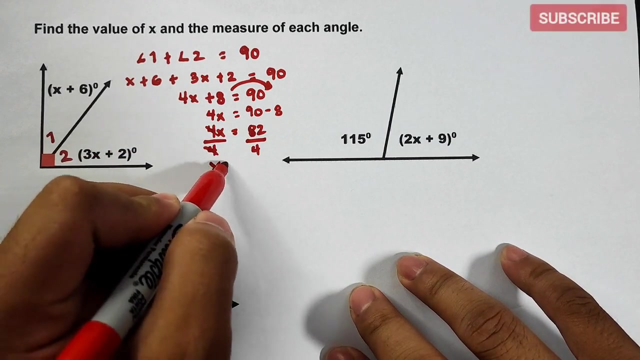 become: 4x is equal to 90 minus 8.. So we have: 4x is equal to 82.. And then what will happen here is that we will divide this by 4.. This one is also by 4.. Cancel, cancel. So, as you can see, we have here x, which is 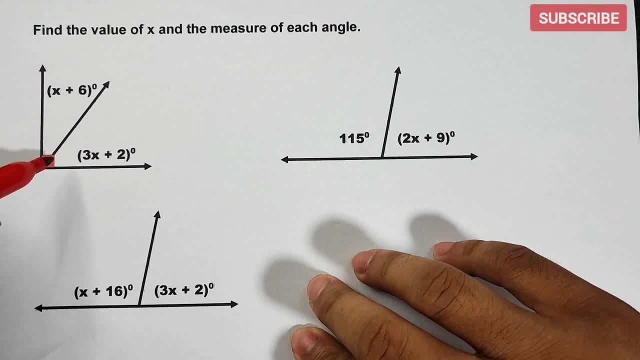 the whole angle or the bigger angle here is a 90 degree angle, meaning we can use the concept of complementary angles because this angle- angle 1 and angle 2, are the same, forming complementary angles. So how are we going to solve this kind of problem? 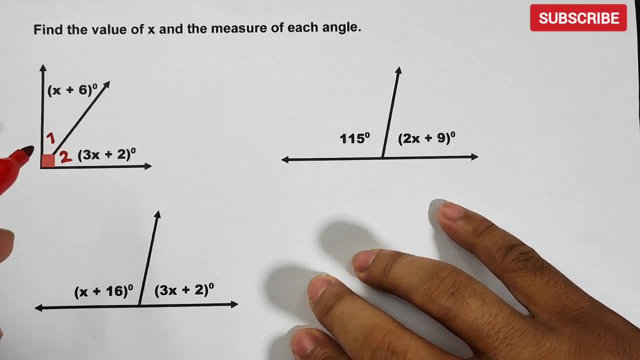 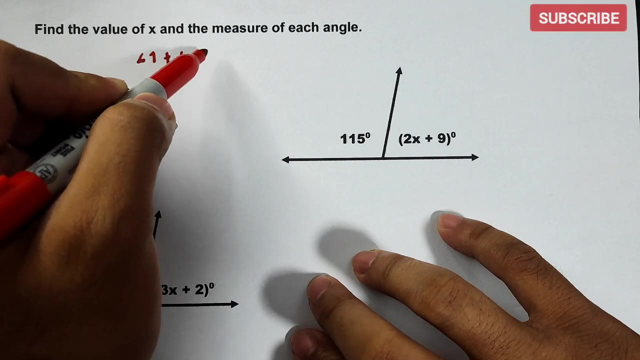 Since they are complementary. the concept is that if the two angles are complementary, meaning the sum of the two angles is equal to 90 degrees. So to solve this, let's create first an equation. We have: angle 1 plus angle 2 is 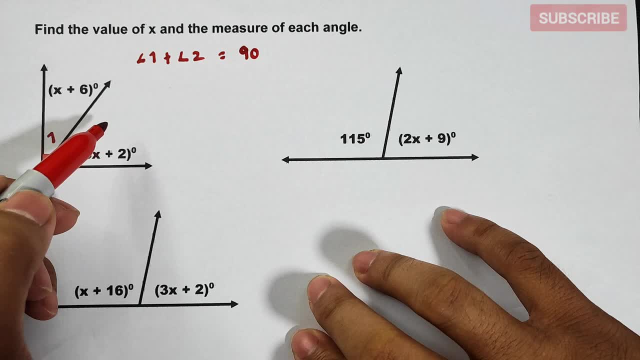 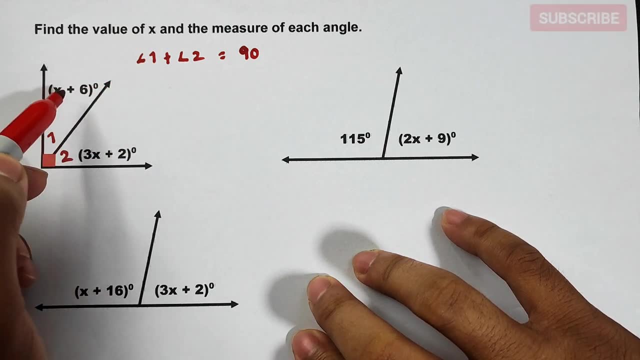 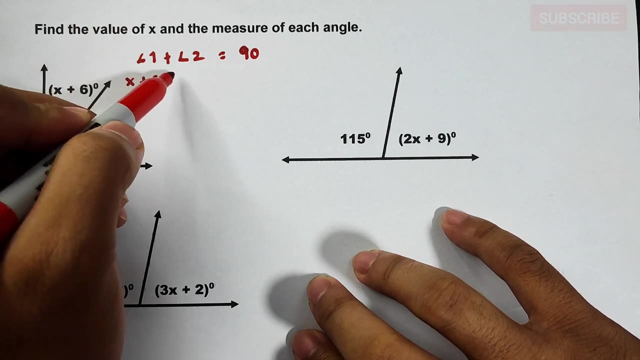 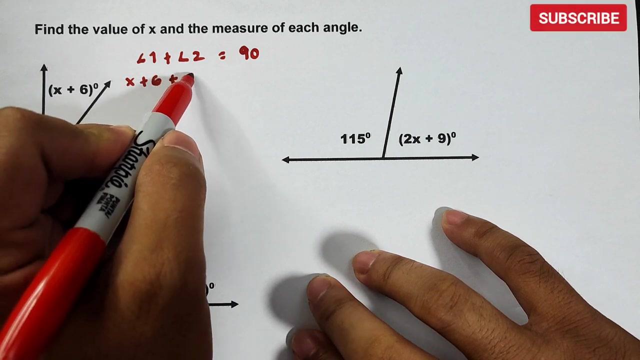 equal to 90 or 90 degrees, Then let's use the expression here represented by this one. Your angle 1 is represented by x plus 1 degree, x plus 6 degrees rather. So let's have x plus 6 plus your angle 2 is represented by 3x plus 2.. We have 3x plus. 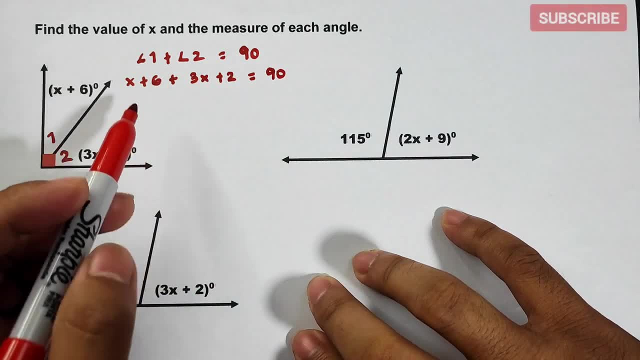 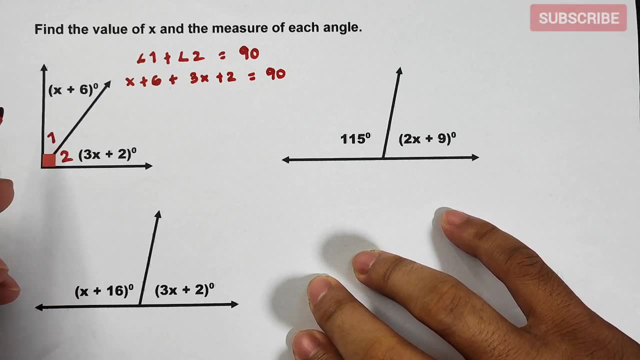 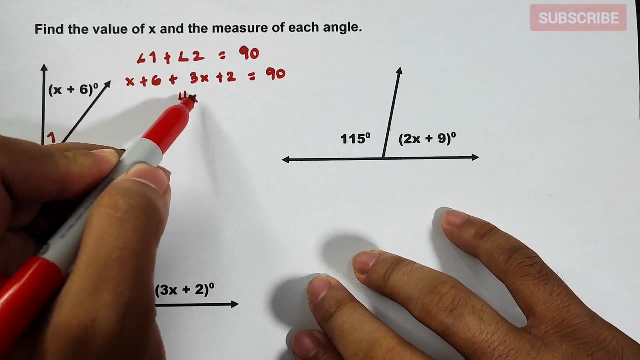 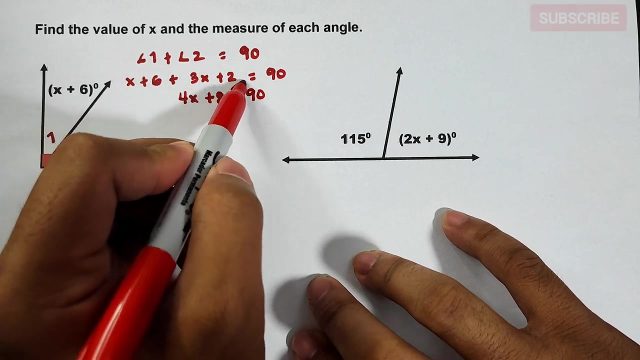 2 is equal to 90.. Our first thing, the first thing we need to do here, guys, is to solve for first for the value of x, for us to find the measurement of these two angles: x plus 3x is 4x, 6 plus 2 is 8 is equal to 90.. Transpose 8 to the other side, it will. 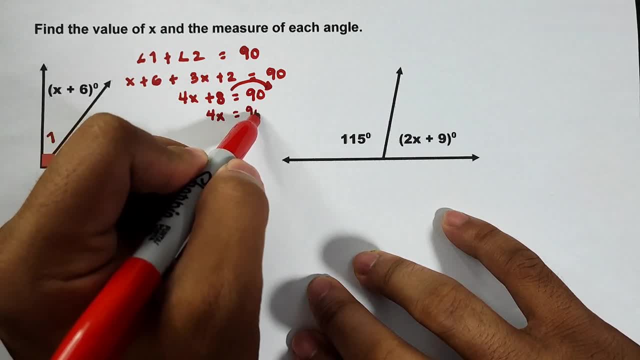 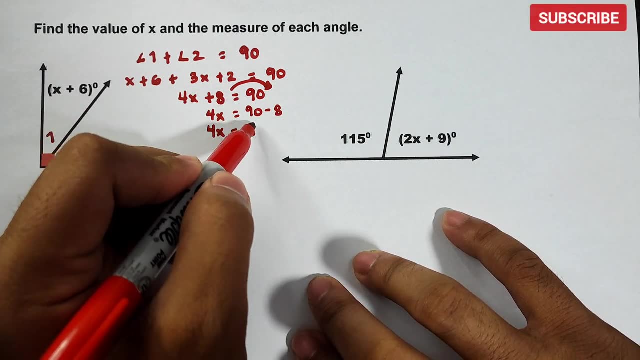 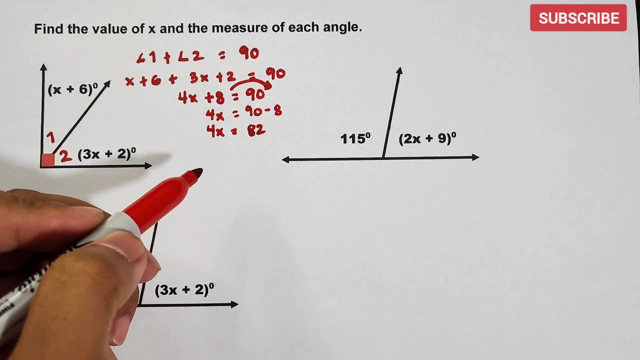 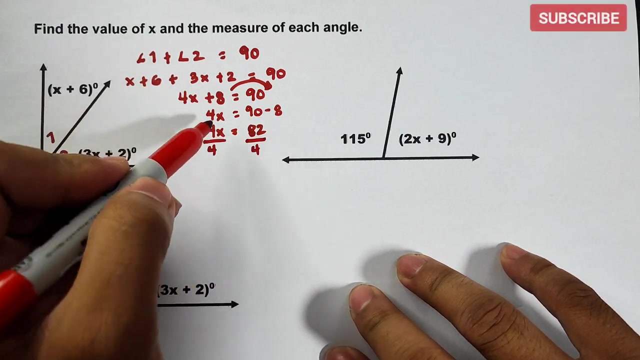 become: 4x is equal to 90 minus 8.. So we have: 4x is equal to 82.. And then We need to find one of these angles, Y and b. What will happen here is that we will divide this by 4.. This one is also died. 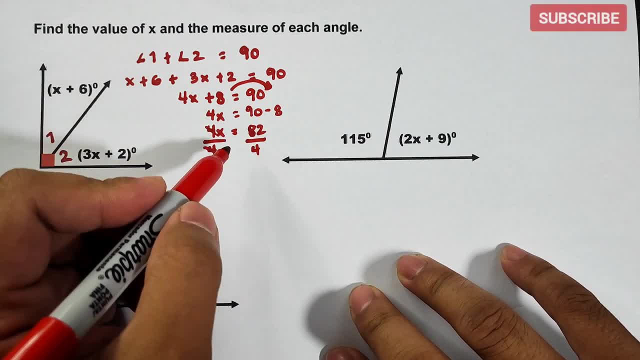 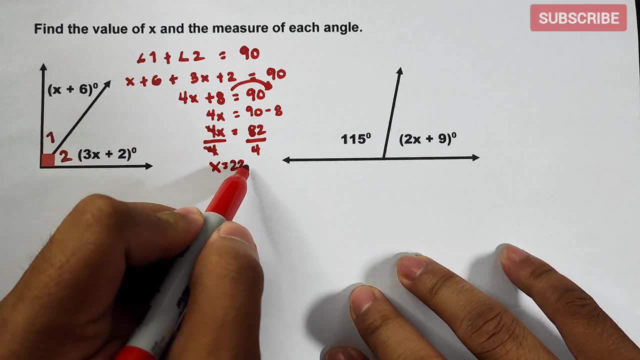 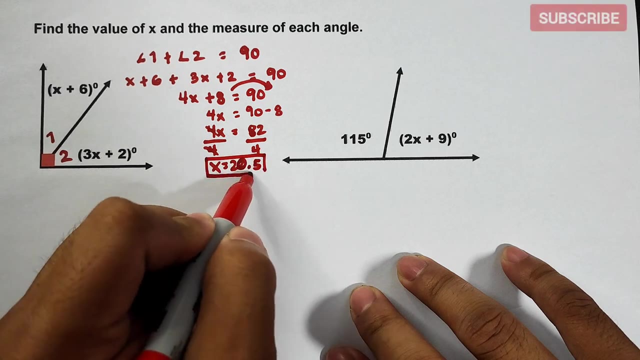 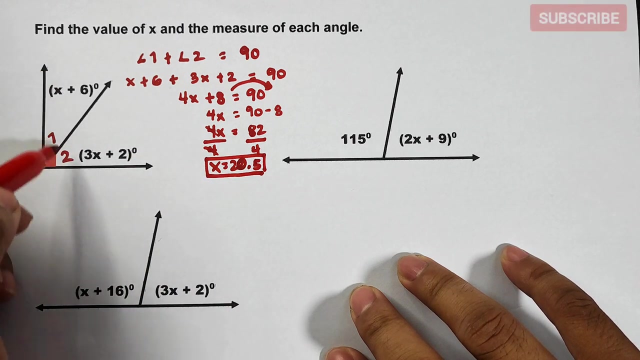 Four Pakas. So cancel, cancel. So, as you can see, Mary is doing X, which is equal to 22 point 20.5. That is the value of x. Now, If x is equal to 20.5, Let's take the value of this. 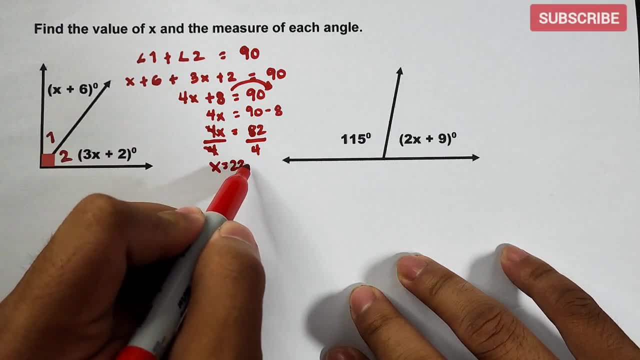 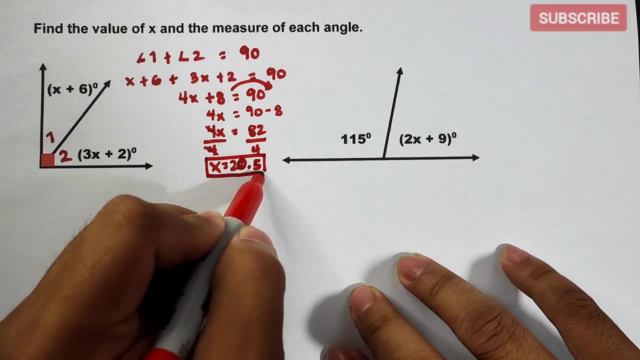 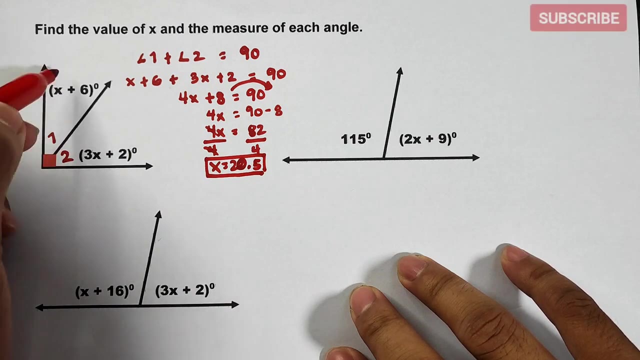 equal to 22.8.. 20.5, That is the value of x. Now, if x is equal to 20.5, let's take the value of this. So this is x plus 6.. x plus 6 degrees. 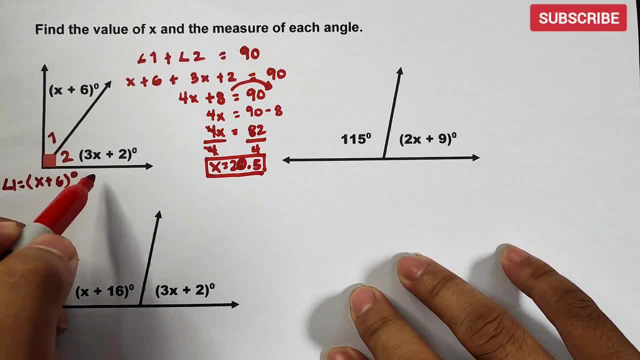 This is angle 1.. So we have 20.5 plus 6 degrees, meaning your angle 1 is 26.5 degrees. So if this is 26.5 degrees, what is not the value of angle 2? Your angle 2. 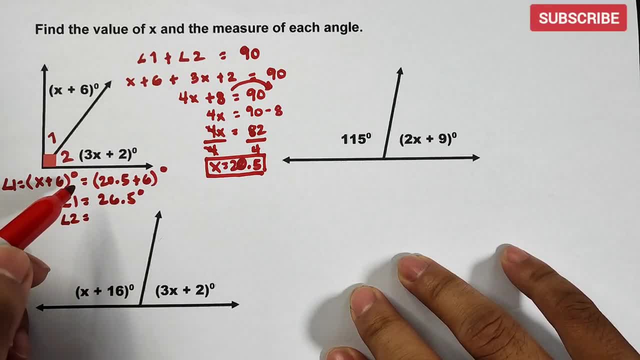 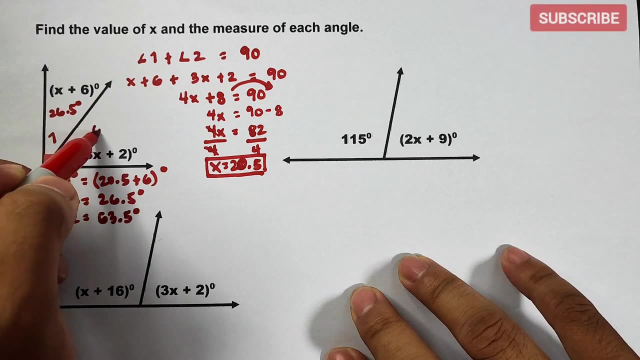 measures. how many? Okay, how many. We have 63.5 degrees. This is 26.5.. This is 66.5 degrees. This is 63.5 degrees. Okay, guys. So let's continue with item number 2.. 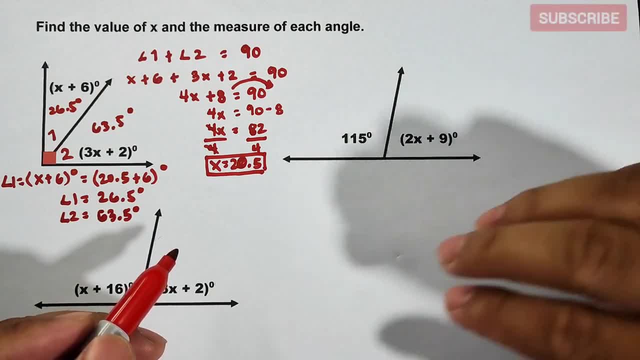 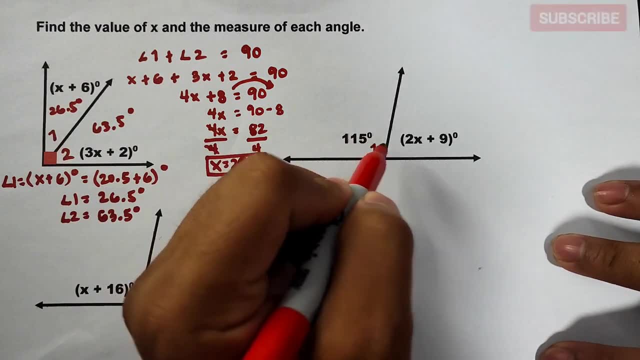 For item number 2,. as you can see, this one is a straight angle. So basically, we will use the concept of supplementary angles. Let's say, for example, this is angle 1 and this is angle 2.. Create a working equation. 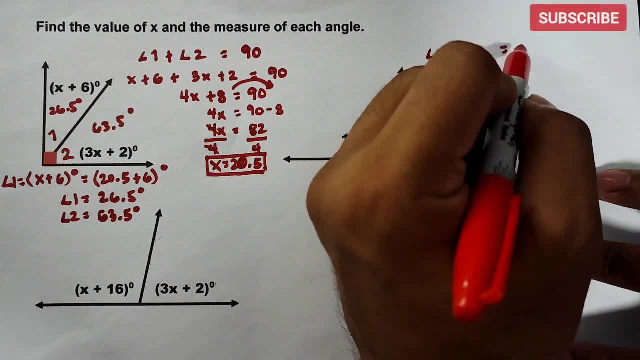 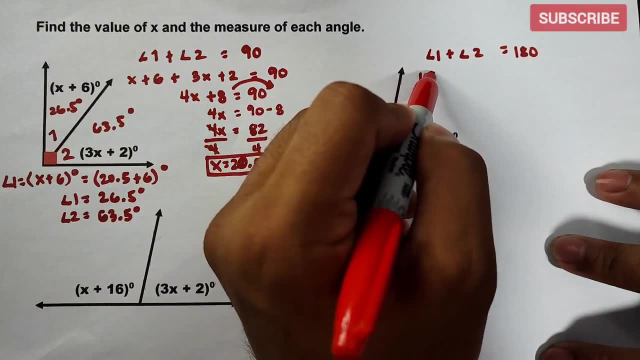 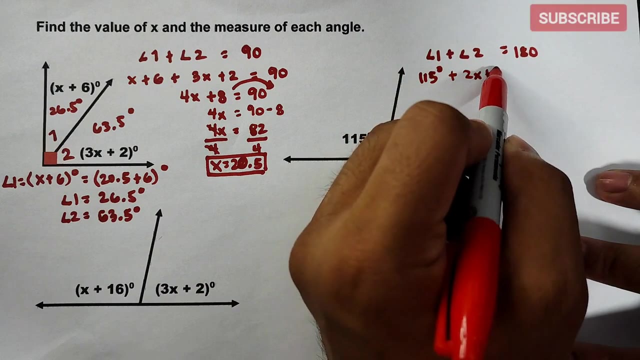 Your angle 1 plus angle 2 is equal to 180 because they are forming supplementary angles. Your angle 1 is 115 degrees, plus your angle 2 is 2x plus 9 is equal to 180.. Combine one and another. 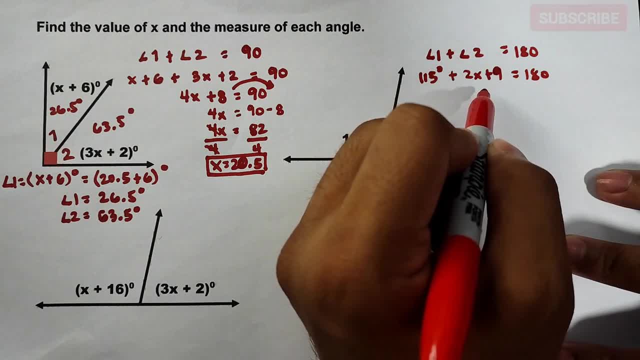 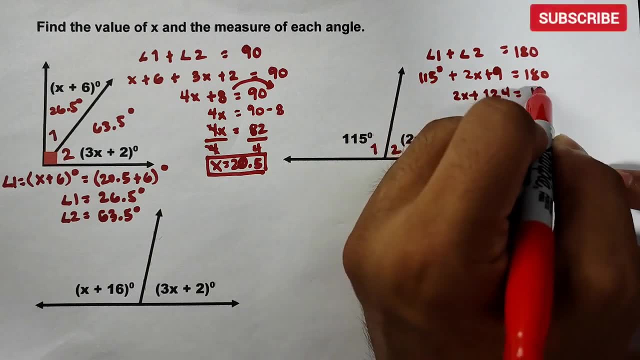 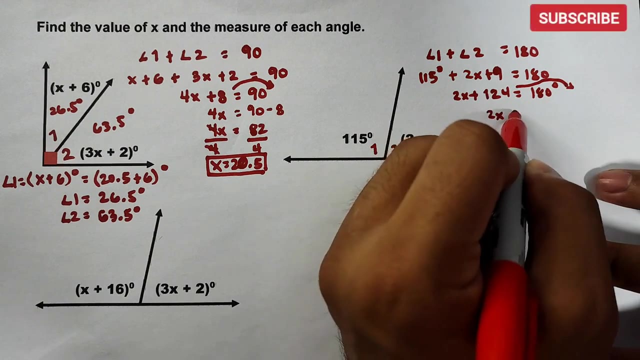 115 plus 9, that is equal to 124.. Plus 2x It's equal to 180 degrees. Transpose 124 to the other side: It will become 2x. It's equal to 180 degrees minus 124 degrees. So this is: 2x is equal to how many 66 degrees To solve for x? because we are asked to solve for x. divide by 2, divide by 2, cancel. cancel. your x is equal to 33 degrees. 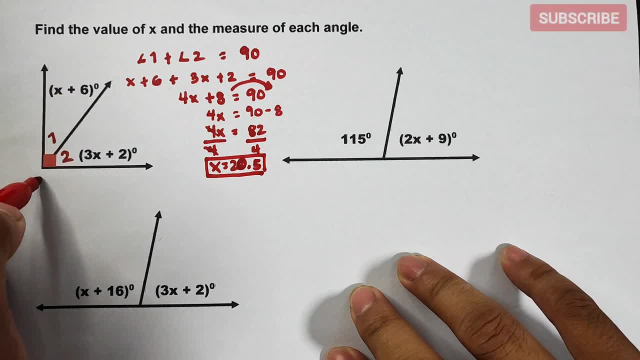 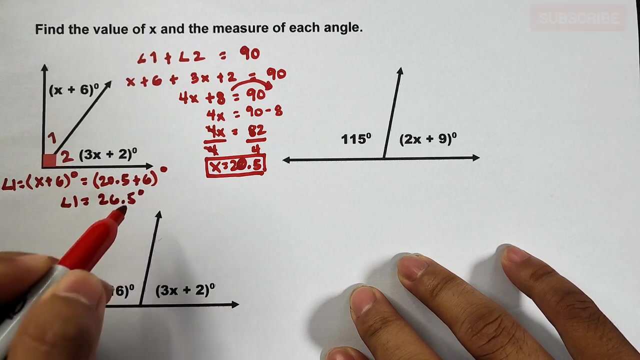 So this is x plus 6, x plus 6 degree. This is angle 1, Angle 1, So we have 20.5 plus 6 degree, Meaning Your angle 1 Is 26.5 Degrees. So if this is 26.5 degrees, 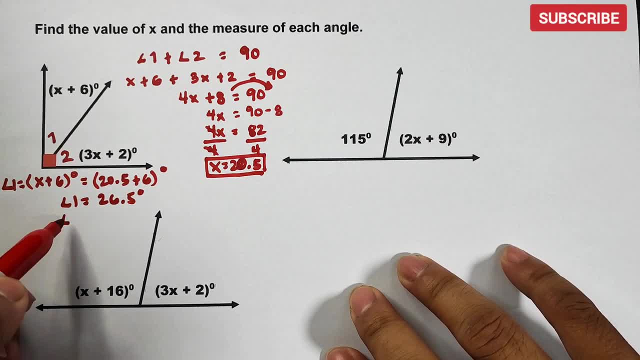 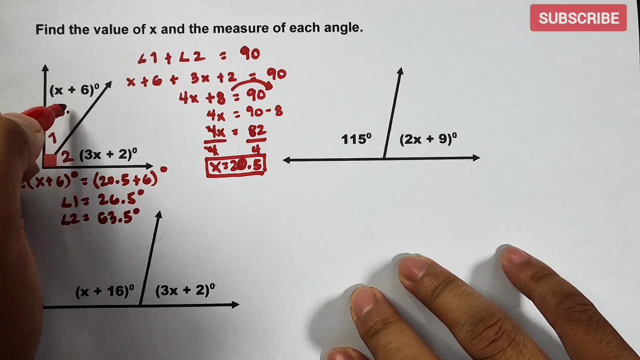 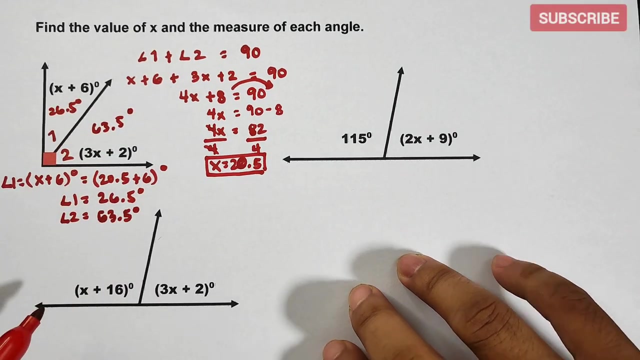 What is not the value of angle 2? Your angle 2 Measures how many- Okay, How many. We have 63.5 Degrees. This is 26.5 Degrees. This is 63.5 Degrees, Okay, guys. So let's continue with item number 2. 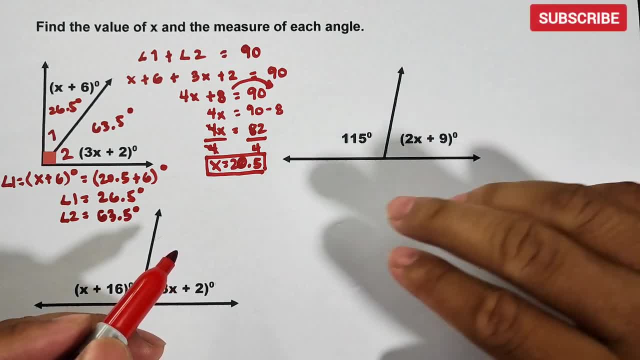 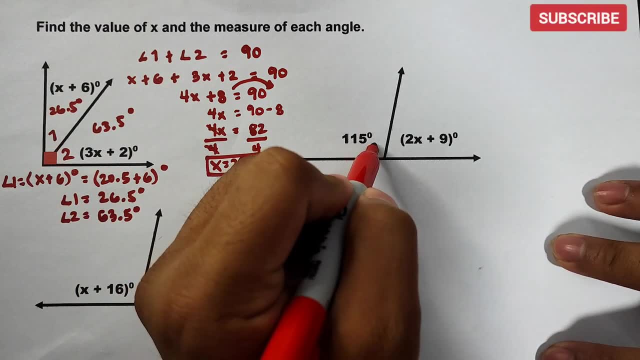 For item number 2, As you can see, this one is a straight angle. So basically, we will use the concept of Supplementary angles. Let's say, for example, This is angle 1 And this is angle 2. Let's create a working equation: Your angle 1. 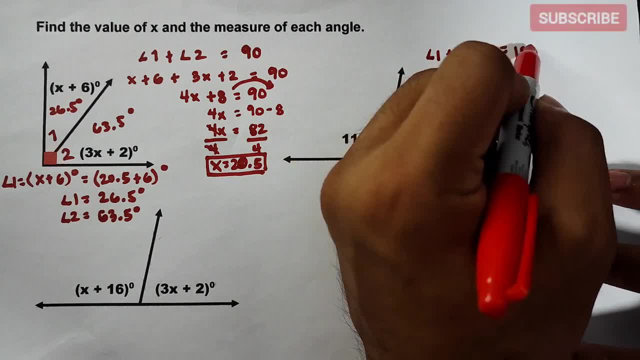 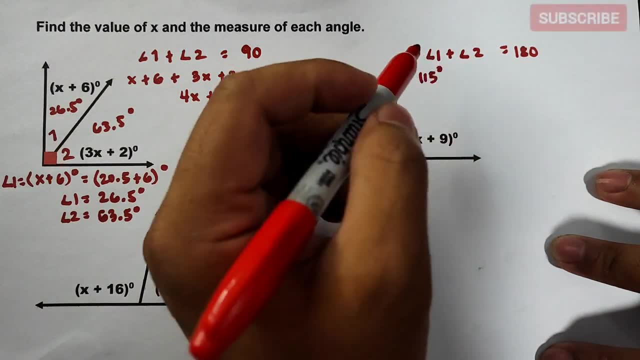 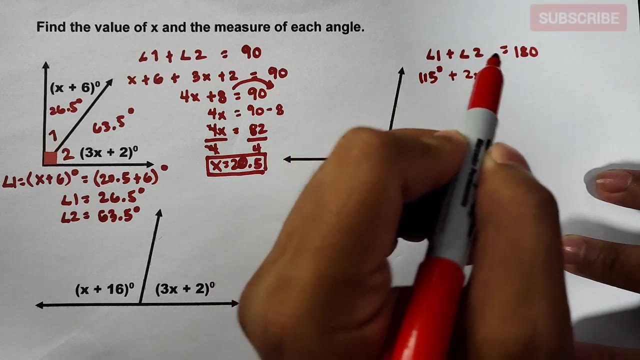 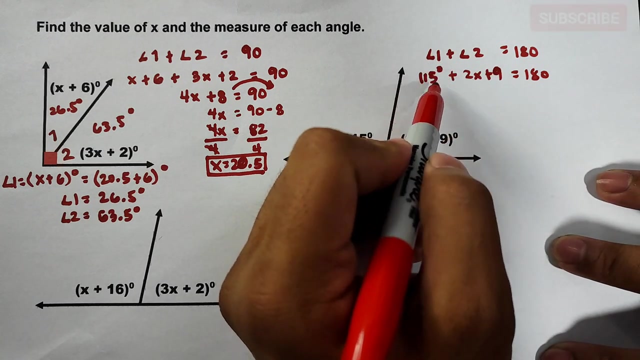 Plus angle 2 Is equal to 180 degrees Because they are forming supplementary angles. Your angle 1 is 115 Degrees Plus Your angle 2 is 2x Plus 9 Is equal to 180. Let's combine them 115 plus 9, That is equal to. 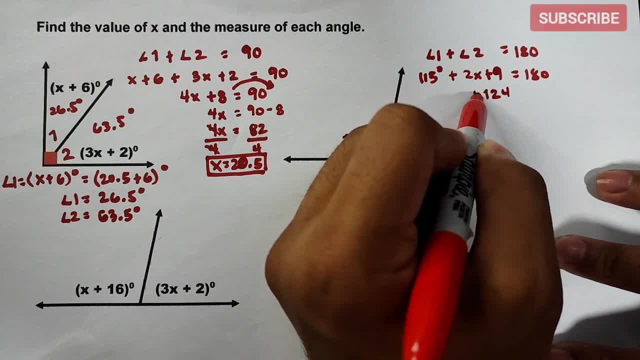 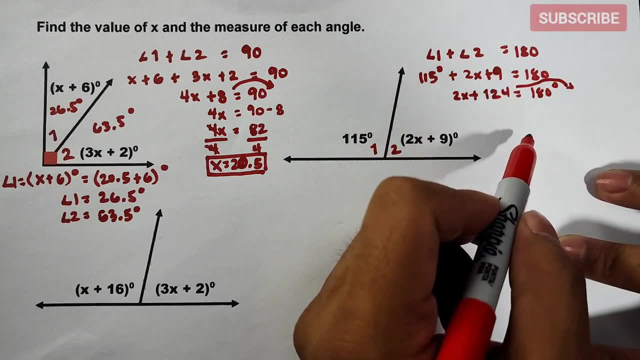 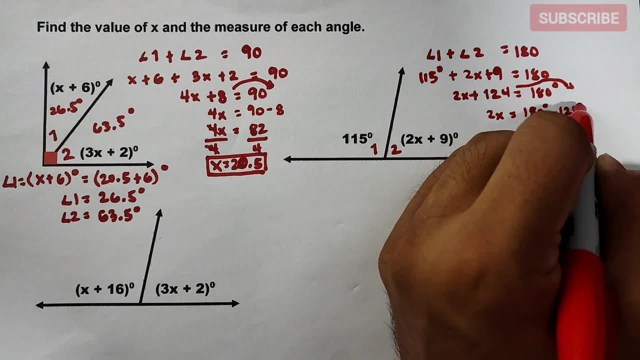 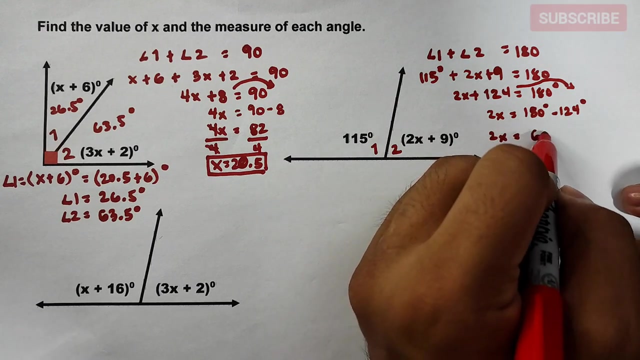 124 Plus 2x Is equal to 180 degrees. Transpose 124 to the other side, It will become: 2x Is equal to 180 degrees Minus 124 degrees. So this is 2x Is equal to How many 66 degrees. 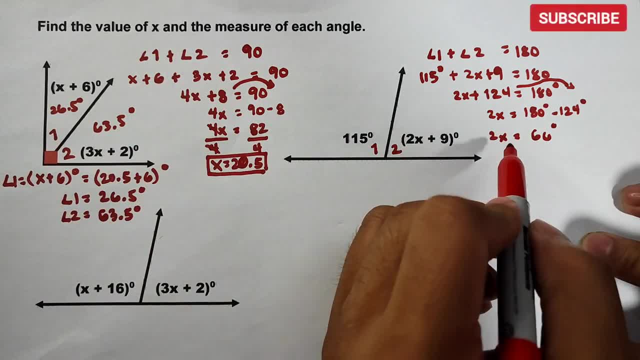 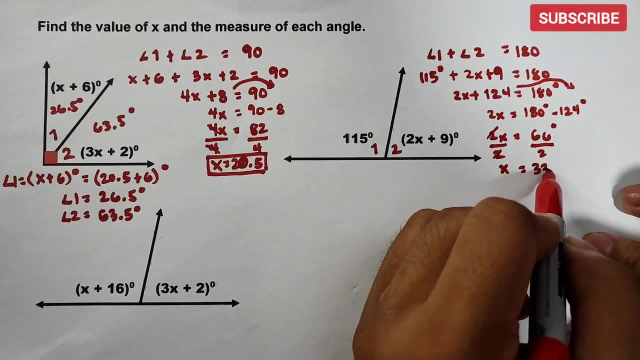 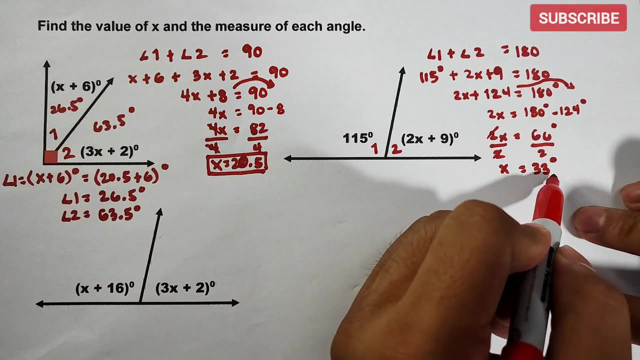 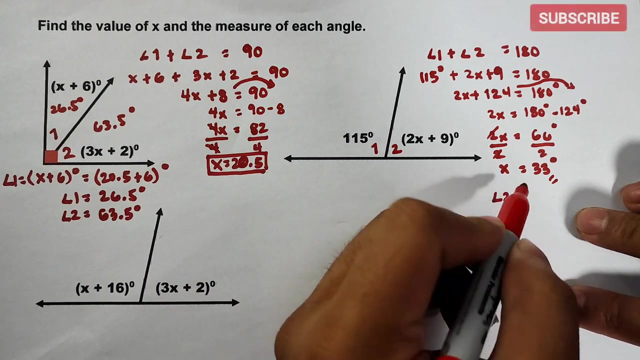 To solve for x, Because we are asked to solve for x. Divide by 2. Divide by 2: Cancel. Cancel. Your x is equal to 33 degrees. Actually, We only need x to find the data, Because If your angle 1 measures 115, Automatically Your angle 2 is: 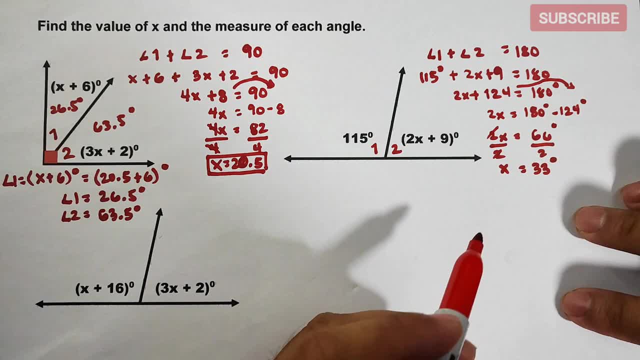 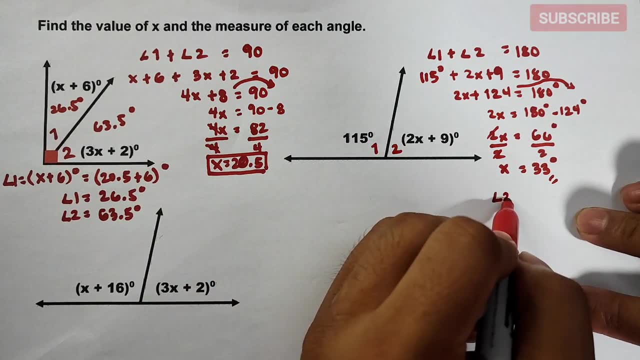 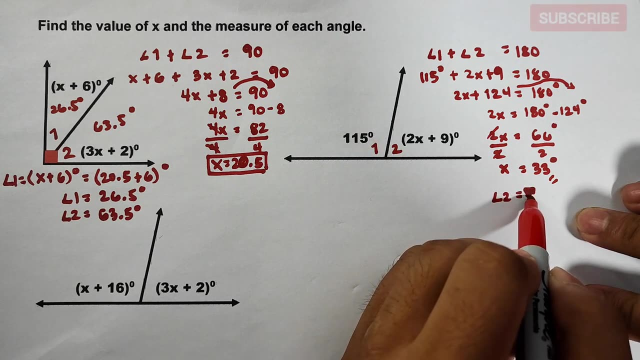 Actually, x is the only thing we need to find in data, Because if your angle 1 measures 115, automatically your angle 2 is how many? That is sorry, 65 degrees. That is the answer for that, Okay. 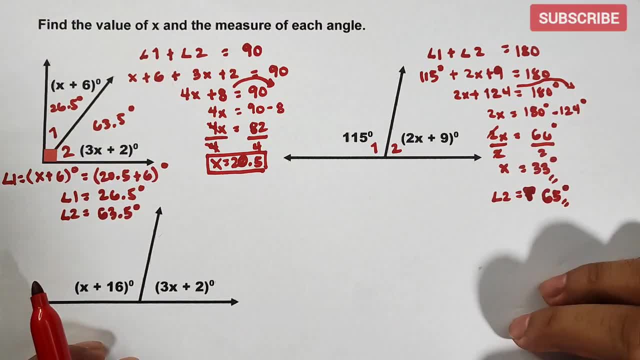 I hope you got this concept. Now let's move on with the next example, So the concept of supplementary angles. So let's add them. This is angle 1 and angle 2.. Let's add them to the rectangle. 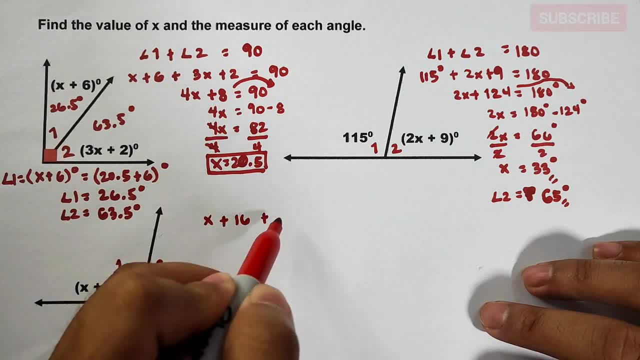 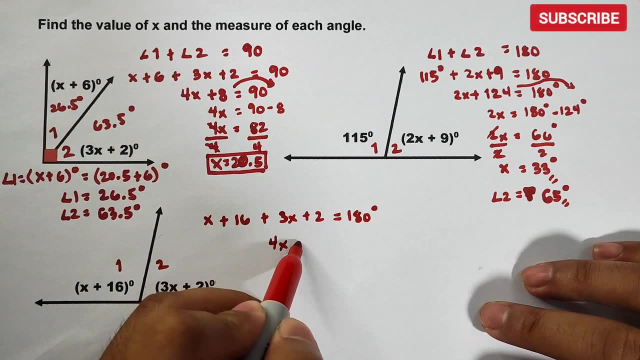 x plus 16 plus 3x plus 2 is equal to 180 degrees. Add them for: x plus 18 is equal to 180 degrees. Okay, Okay. Now let's transpose this to the other side. This is 4x. 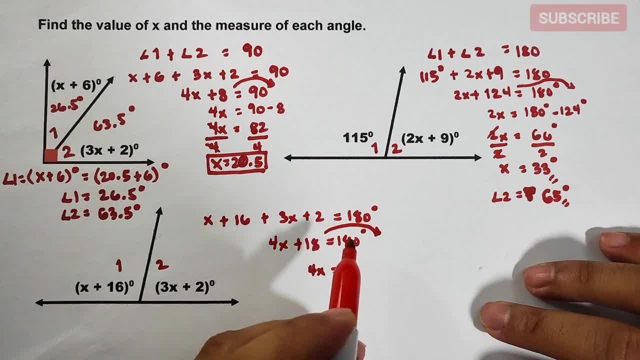 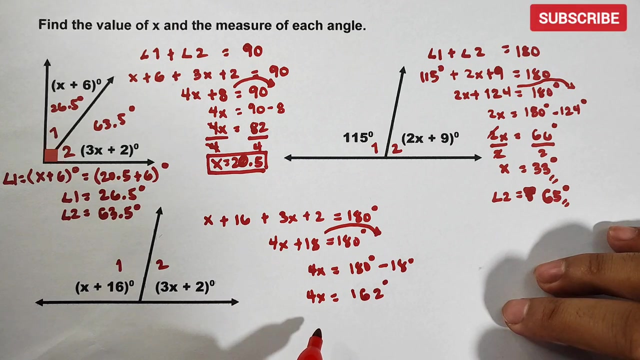 is equal to how many 180 degrees minus 18 degrees. So you have: 4x is equal to how many 162 degrees. So what will happen here? We'll have: 2x is equal to 180 degrees. 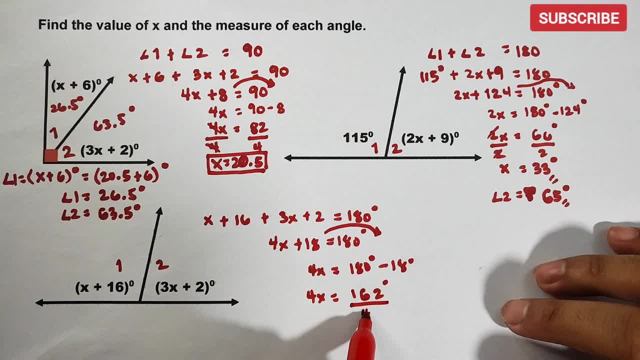 Okay, So divide both sides by 4.. As you can see, it is not the whole number. So your x here is equal to 40.5.. This is the value of our x. What about the measurement of angle 1?? 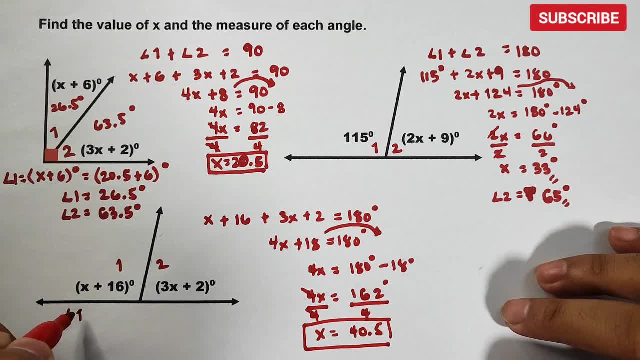 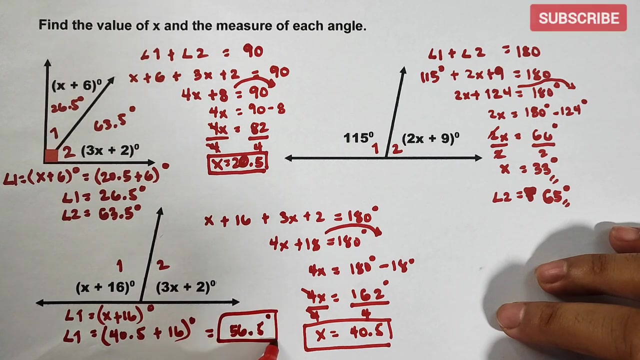 Let's just find angle 1.. Your angle 1 is equal to x plus 16 degrees. substitute natin yung value ng x, 40.5 plus 16 degrees, meaning your angle one is equal to 56.5 degrees. okay, if this is 56.5 degrees. 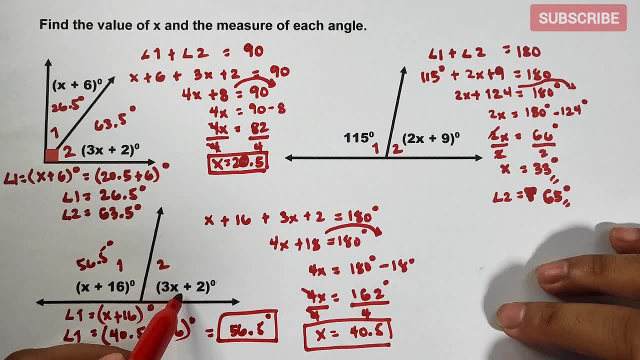 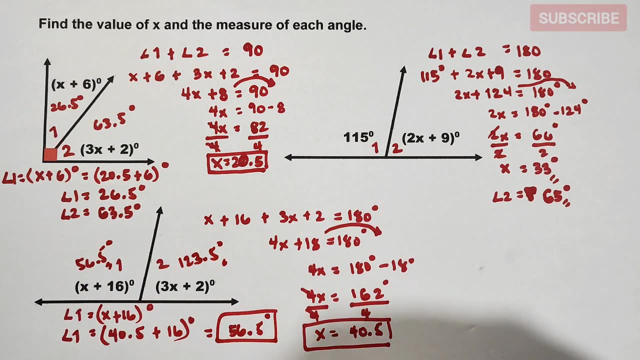 what is the value of this? this one is 123.5 degrees. yun yung angle to natin. so i hope, guys, you learned something from this video. medyo congested lang yung paper natin, dahil sya na maraming solution. 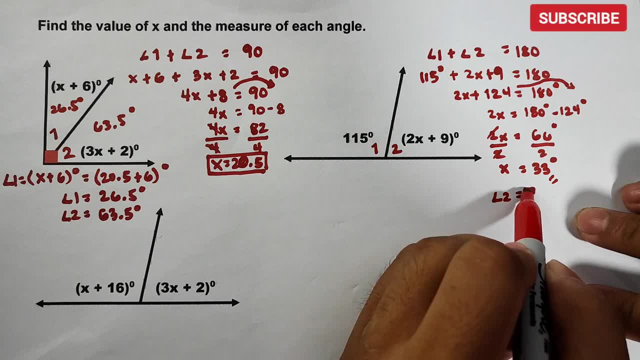 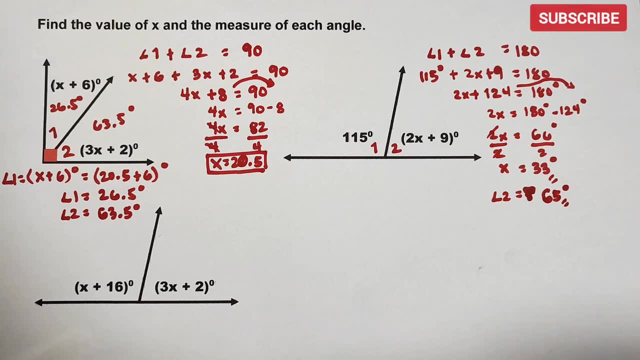 How many? That is Sorry, 65 degrees. That is the answer for that. Okay, I hope that you got this concept. Now let's move on with the next example. So the concept is supplementary angles. So let's add them. This is angle 1, Angle 2: Let's add them to the rectangle. 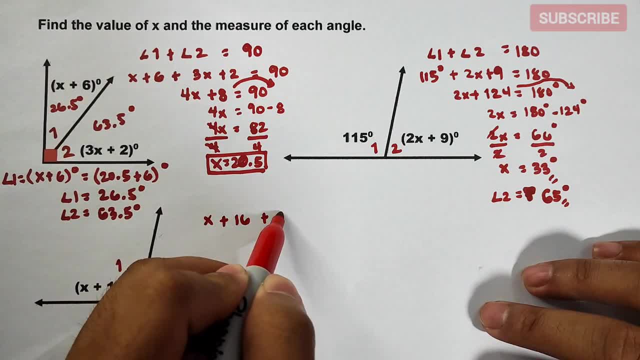 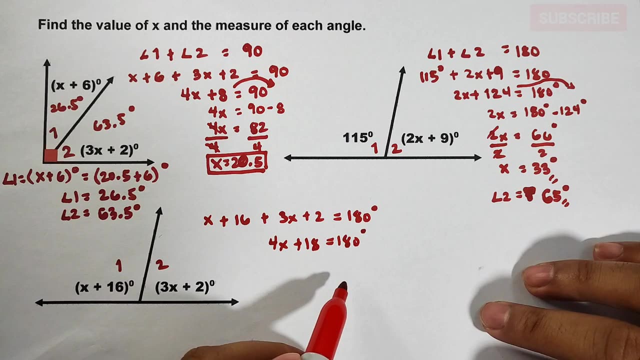 x plus 16 Plus 3x plus 2 Is equal to 180 degrees. Add them: 4x Plus 18 Is equal to 180 degrees. Okay, Now let's transpose this to the other side. This is: 4x Is equal to How many? 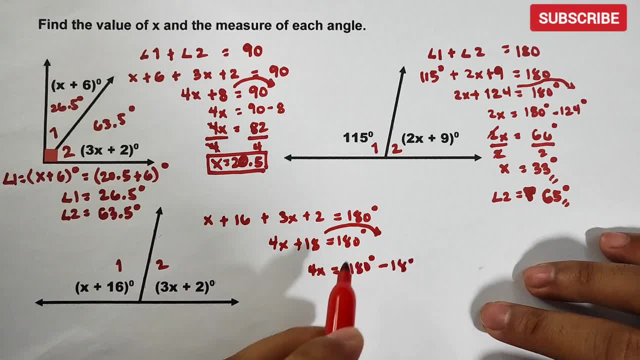 180 degrees Minus 18 degrees, So you have 4x is equal to How many 162 degrees. So what will happen here? Okay, So divide both sides By 4 By 4. As you can see, It will not be the whole number. So your x here. 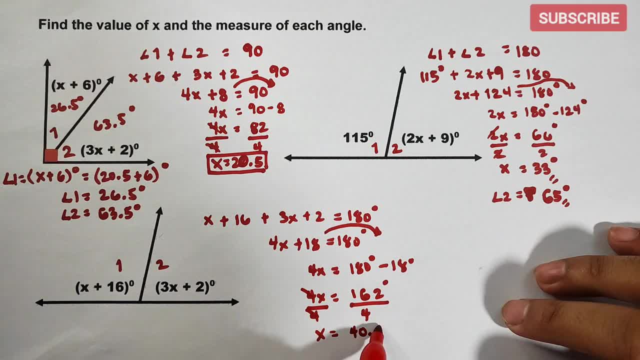 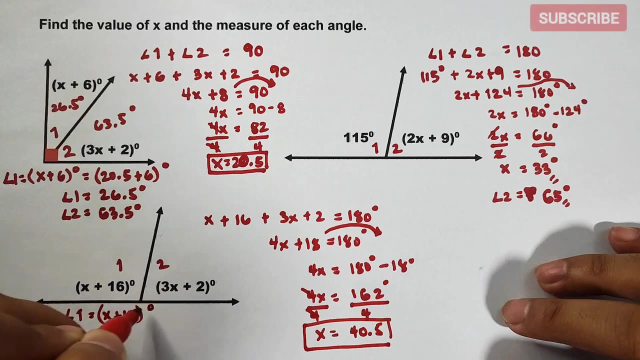 Is equal to 40.5. This is the value of our x. What about The measurement of angle 1? We will just find angle 1. Your angle 1 is equal to X plus 16 degrees. Let's substitute the value of X: It's 40.5 plus 16 degrees. 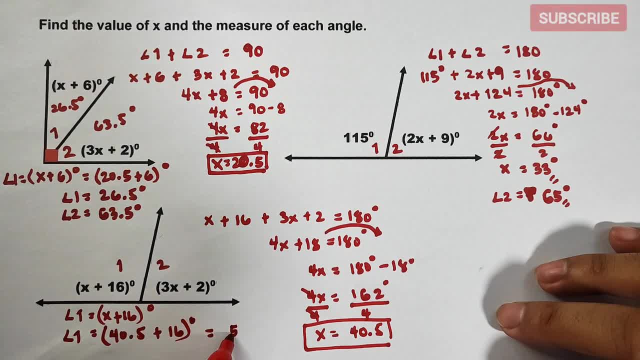 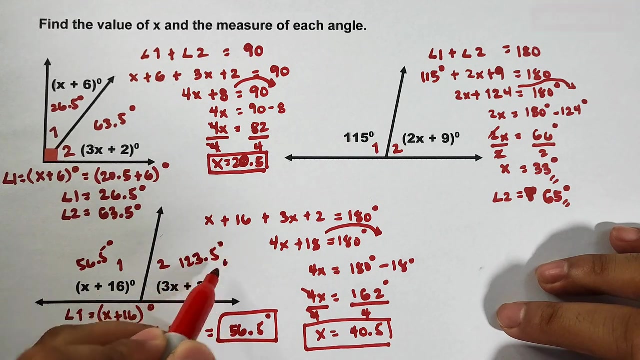 Meaning your angle 1 is equal to 56.5 degrees. Okay, if this is 56.5 degrees, what is the value of this? This one is 123.5 degrees. That's our angle 2.. So I hope, guys, you learned something from this video. Our paper is a bit congested. 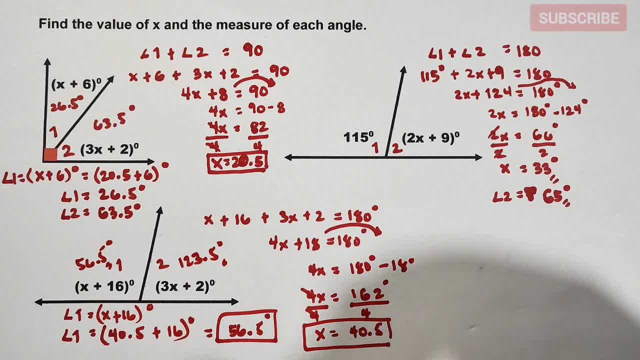 because it has a lot of solutions. By the way, if you're new to my channel, don't forget to like and subscribe, but also hit the bell button for you to be updated on our latest uploads. Again, it's me, Teacher Goyen.